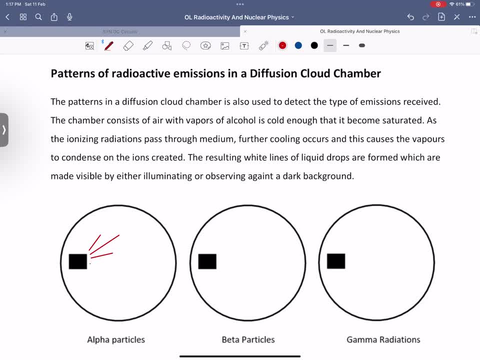 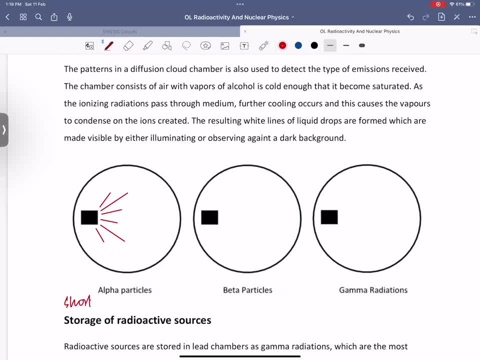 Please add punctuation in the appropriate places. Please add punctuation in the appropriate places. it forms short tracks, but straight ones. straight because alpha is a very heavy particle. these alcohol vapors. it's not easy for these alcohol vapors to deflect an alpha particle from its track. 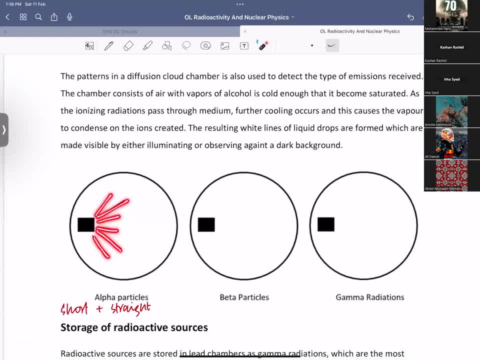 the alpha particle comes out straight, but it can travel a small distance, after which you know that alpha doesn't remain as alpha. after that we talk about beta particles. about beta particles the tracks are not straight, because beta particles are electrons, so their motion is not that rigid. 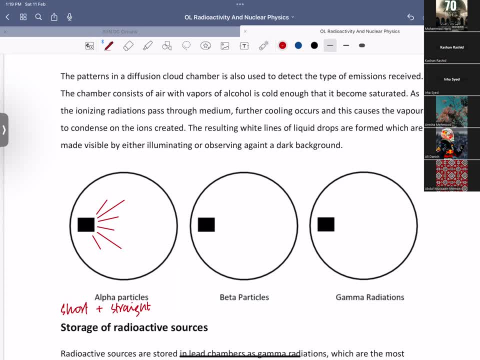 their motion is affected because the tracks are not straight. alcohol's saturated vapors condenses easily when they get ionized, so their tracks more clear and visible. these tracks are comparatively longer but more wavy. see, they are long, they are thin. they are long and slightly round. 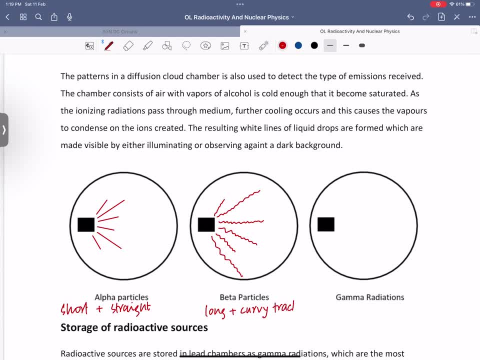 Plus curvy tracks Because beta particles are generally like affected by the alcohol vapors in the surrounding. They deflect back and forth Gamma radiations, do very little ionize Because they don't have any charge, So their tracks are also not that good. 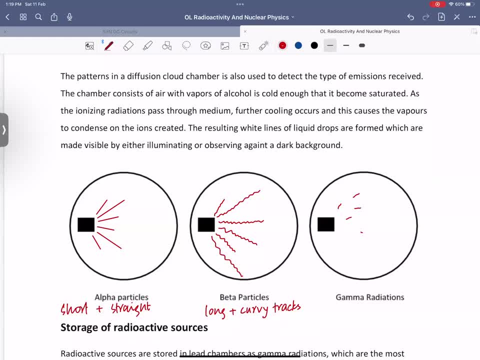 Gamma radiations are generally like a little bit If there is any ionize. So if you see a little bit of track, then it is seen. So these types of gamma radiations have tracks. They are very short And broken, Plus curvy. 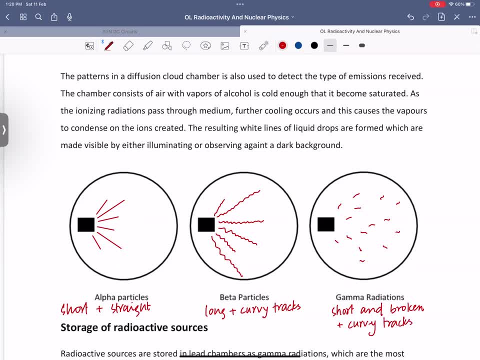 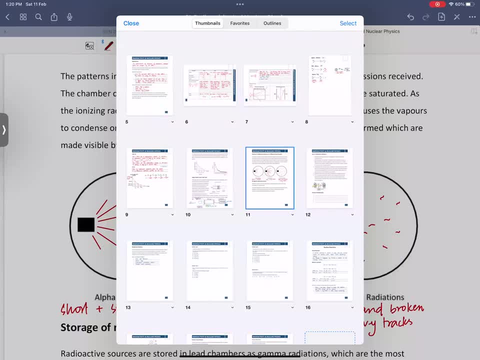 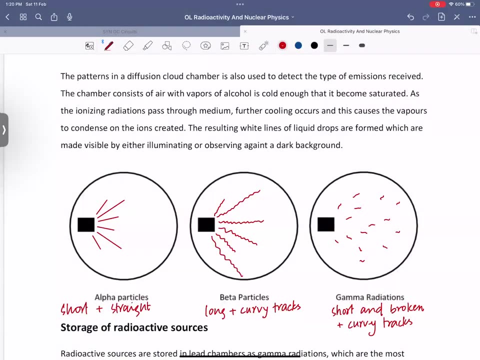 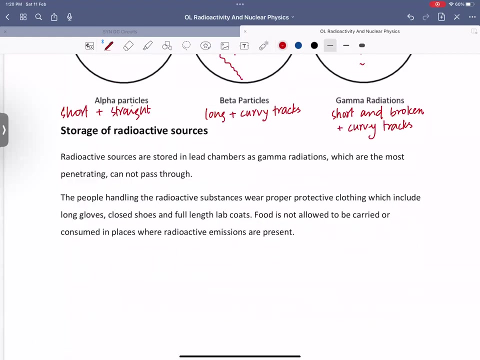 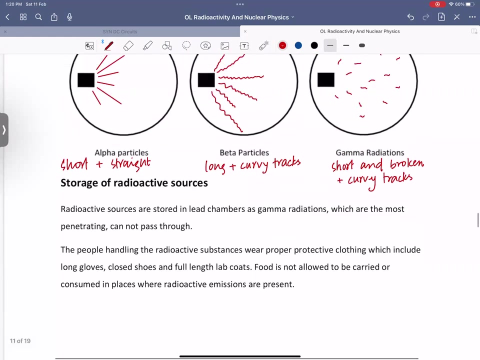 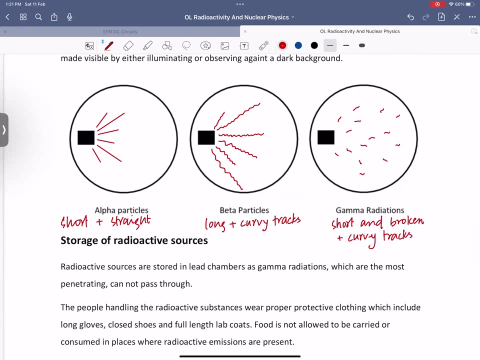 This is the recognition of gamma radiations, That your source was emitting gamma. This is the recognition of gamma radiations. This is the recognition of gamma radiations As it is with them. So we usually keep our radioactive samples Not in like open air. 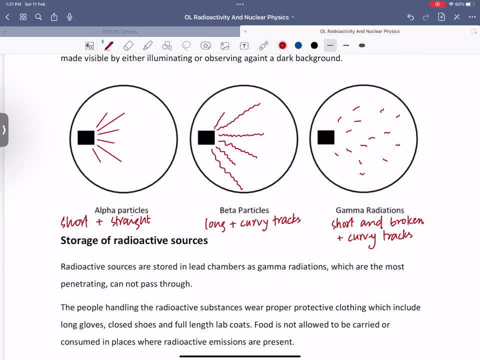 We keep it in a lead block. So about lead? We all know that it ensures none of the radiations actually are able to escape. It stops alpha beta gamma. So a 4 cm or 5 cm thick lead block Ensures that whatever is inside, 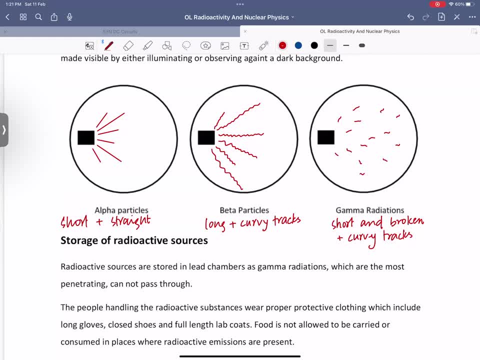 Is not able to come out of. So we always keep our radioactive samples in lead In lead lined blocks. Secondly, We also ensure that we don't carry any eatables or drinkables in the vicinity Where there are radioactive samples, Because our food can get contaminated. 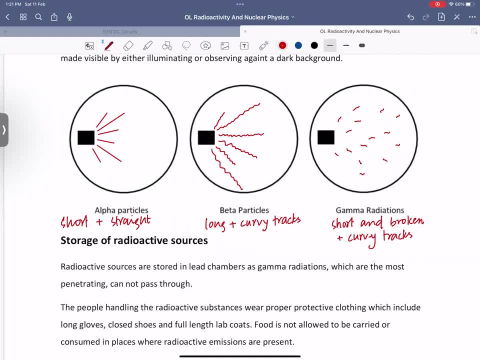 We wear proper clothing, We wear gloves. We don't handle radioactive atoms just by holding with our hands. For that we use clippers etc. We use proper handles etc. We use them to hold it in one place or another. To hold it in one place. 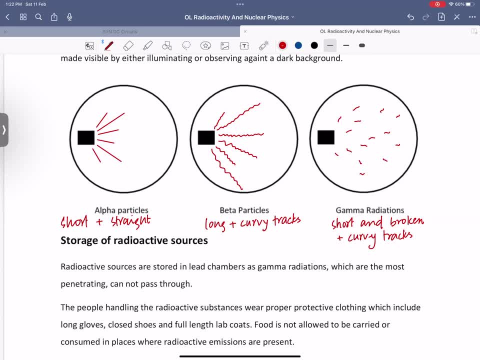 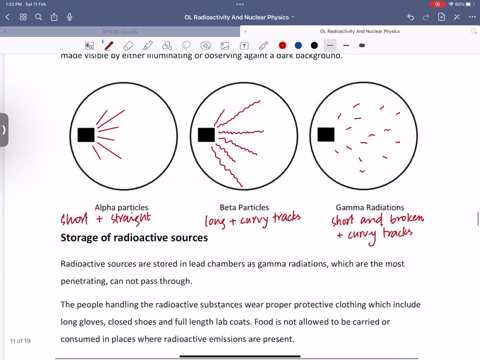 We use masks, etc. So that we don't get excessive exposure of such types of radioactive substances. Something or the other happens, But at least we don't get excessive exposure. Now let's go on. There are a few uses of radioactive substances. 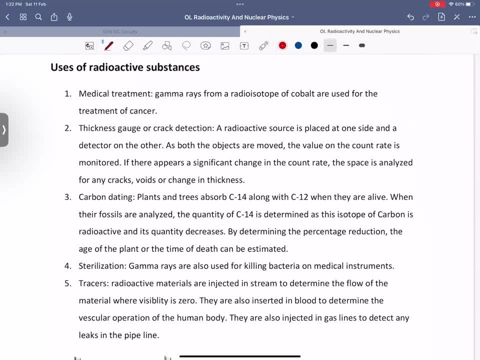 About which I'm not particular about any element Or so, But yes, Generally Many radioactive samples can be used At different places, And for that I want you guys to give These few uses a read And see if you can imagine. 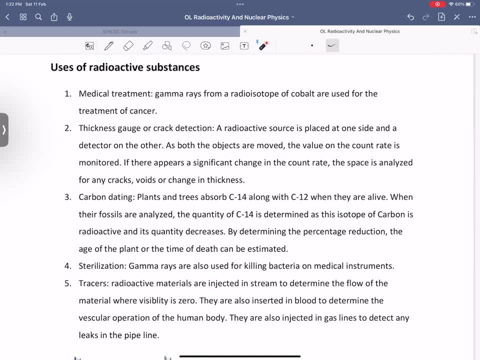 Okay, fine, How are these radiations generally used? Just say, we all know that gamma radiations are there In chemotherapy to treat cancerous cells In human body. Gamma radiations are exposed, So there is radioactive radiation, But in its medical treatment. 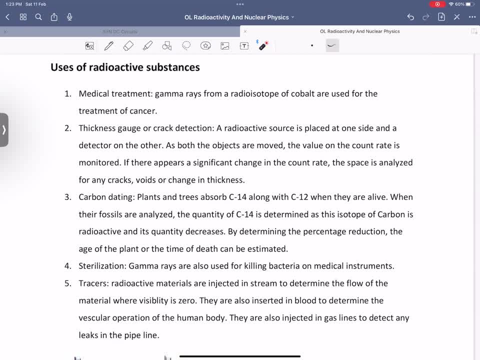 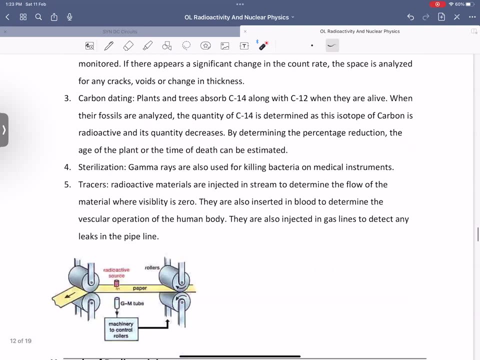 Its application comes So You can use a thickness gauge Or crack detection In the radioactive samples, Because it happens that you have Any particular paper If it is passing from here, You have a radioactive source And a GM tube beneath it. 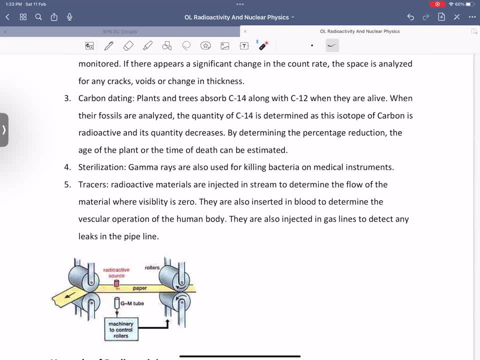 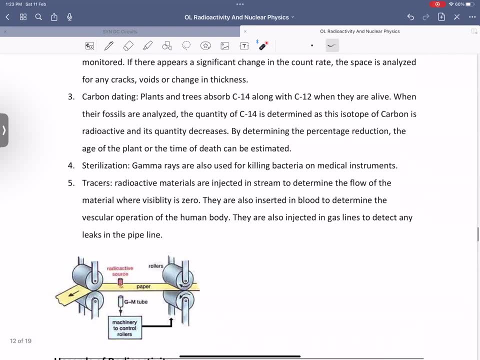 And that paper is being passed from the middle, The thickness of which is being controlled Using rollers. So if, by chance, it happens That the paper gets thick, Then it will happen that the radiation That is passing through it Will start to reduce. 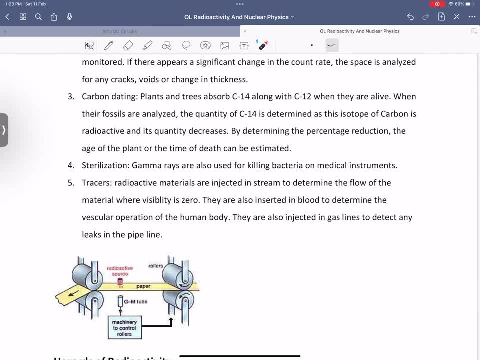 Because thick paper Can stop more radiation. The result will be that the radiation That is passing through it Will drop in quantity, So your reading will start to fall From here. you usually automate That if reading Comes down from this particular value. 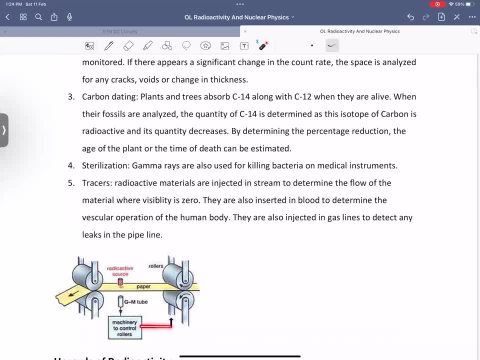 That means the paper has become too thick. So it sends a command To the rollers So they come closer And start to thin the paper. So you can control this Through computer programs, That the product that is being made, How the thickness of it, varies. 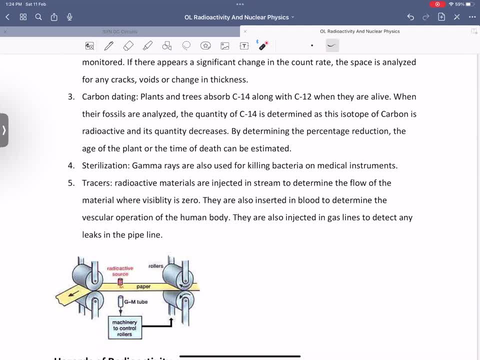 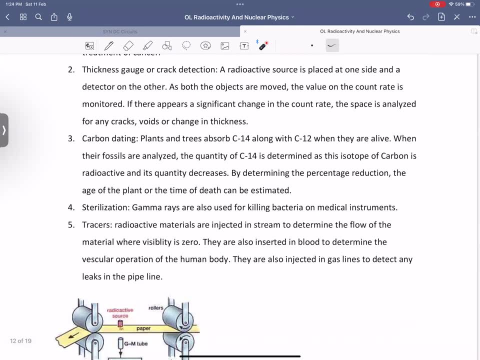 This can also be used for metals. By looking at this paper example, I have just explained it to you. Similarly, it is called something Carbon dating. In other words, It is also called archaeological dating, Through which you figure out That if you are getting any prehistoric stuff, 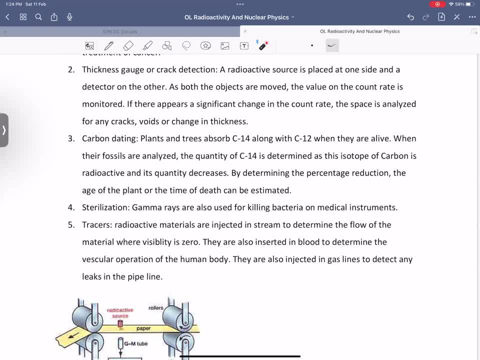 Or any artifact That you are getting? Then how many years old is it So to find out that You use a particular atom, That is, an isotope of carbon Called carbon 14.? So carbon 14. Is basically an isotope of carbon. 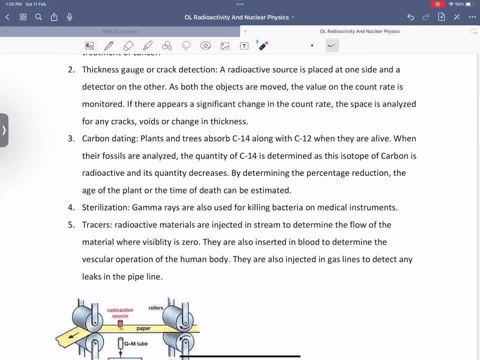 In which Normal carbon Has more than two neutrons, So its nucleus is radioactive. It is unstable. So plants and trees: They actually absorb C14. And they are alive And when their fossils are analyzed The quantity of C14 is determined. 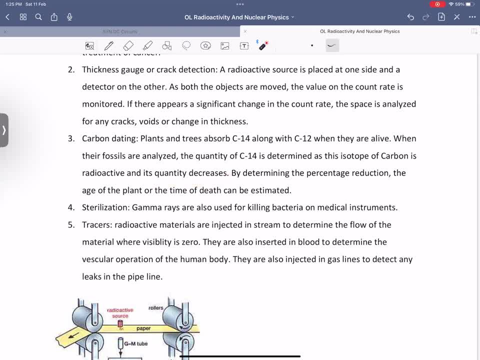 As this isotope of carbon is radioactive And its quantity decreases With time. The carbon content in any living organism, The percentage of carbon 14.. Is normally This much? Normally, So this percentage, Normally, And when it is dropped? 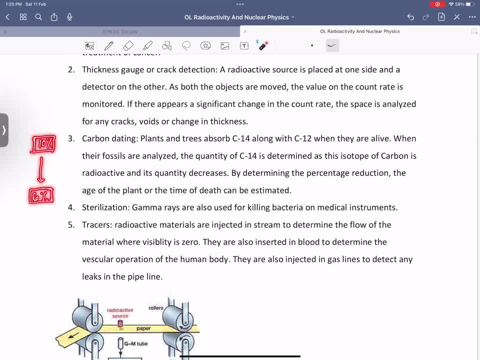 This much is there. The percentage should be 10% And now it is 6%, So you can use this To find out how long For time is spent Before this Percentage drops from 10 to 6.. Through this, you can guess. 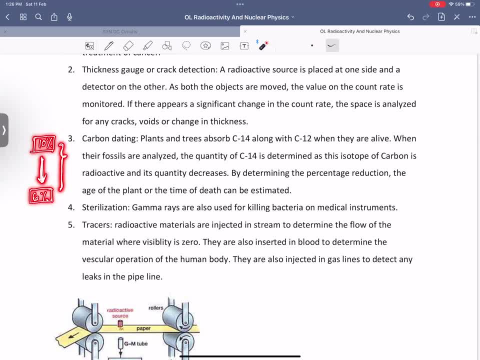 like a million years or, for example, these many hundred years or thousand years in which you have this carbon percentage from here to here, And from here you get to know that this mammal or this artifact or any living organism was actually these many years old. 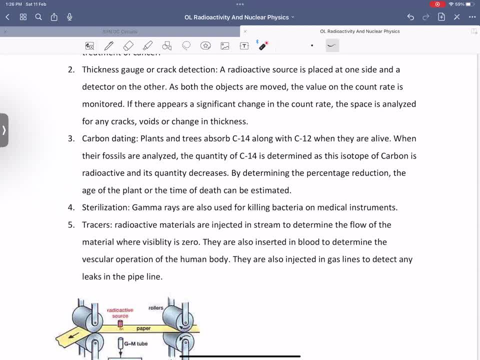 The actions about dinosaurs and other things were done from this perspective. Is my voice lagging, My children? because Hamza's message is that my voice is lagging. If it is, then tell me. Is it clear, Hamza? check your internet. 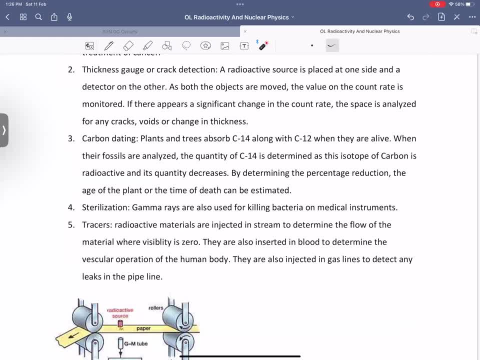 It may be that I am clocking it, Okay. Okay, Gamma radiation is also sterilized for germ-killing, but in a very controlled quantity. It is not that you start getting full exposure from gamma radiation. You don't do that. 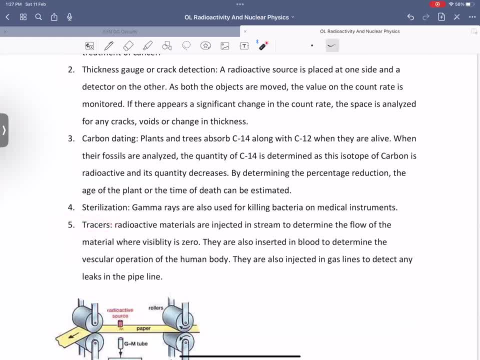 And the same way. tracers. What are tracers? Tracers are such things from which a signal is coming out and you can track the movement of that thing. You can track the movement of that thing. There are trackers installed in our car. 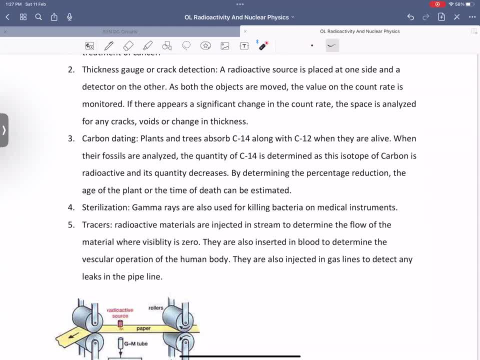 If not, then we can continuously find out where our car is going. So in Tracers there are some molecules that are injected into our body and they attach to a radioactive atom So that it continuously gets radiations. And wherever those molecules go, 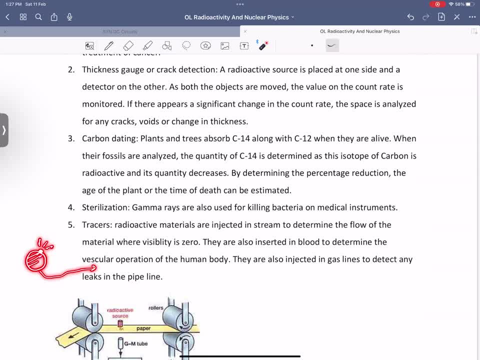 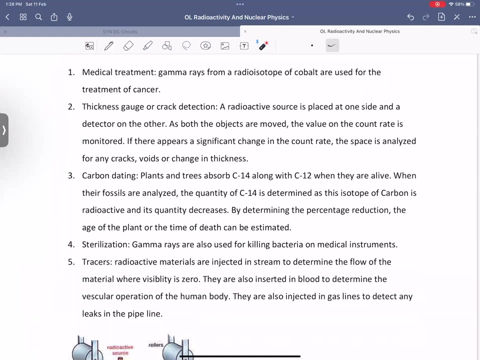 the radiation that is released from that can tell us that this molecule is now present in the body. So this is used to do internal evaluations in the human body. So I gave this explanation. I would like you to read these five points once So that I can take it further. 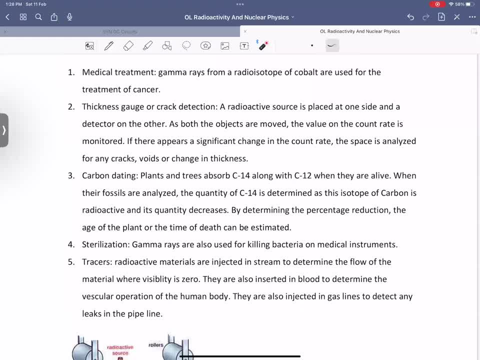 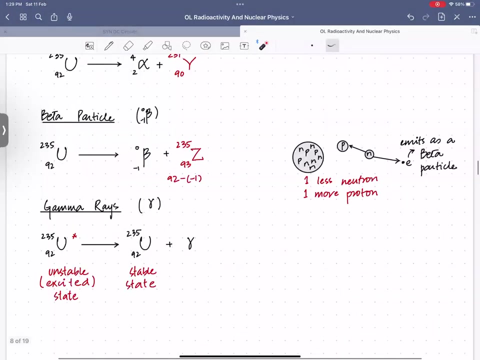 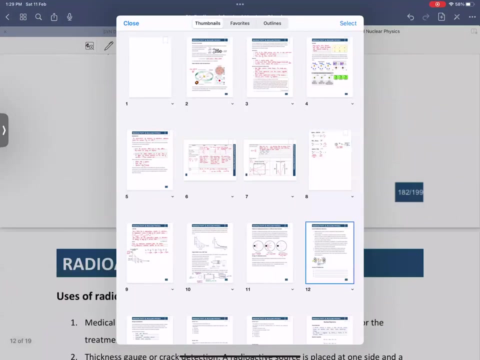 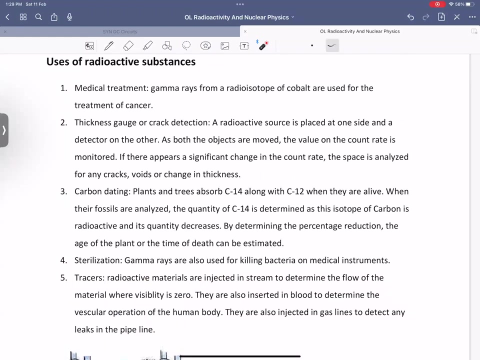 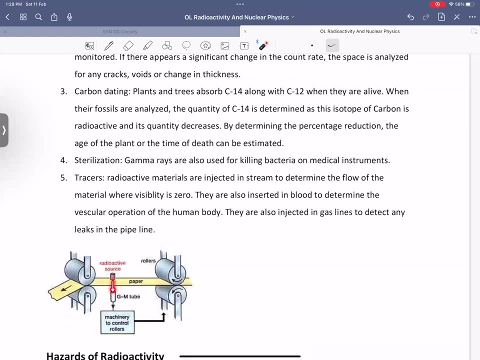 Thank you, We have done equations of emission. We did that, Thank you. Thank you To explain equations of emission. Point two, I use thickness gauge. In the thickness gauge you have radiation passing through a particular metal or sheet of paper. 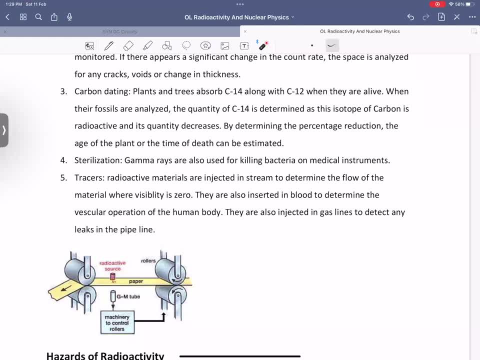 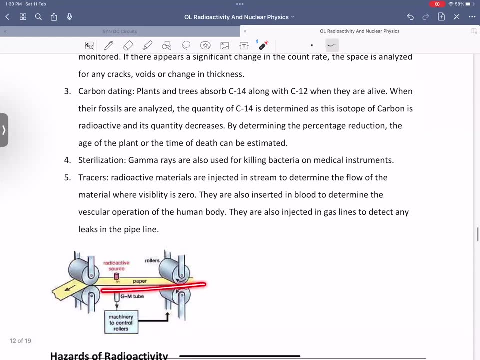 You have to control its thickness by saying what? So if paper gets more thick, then readings will fall. The paper will not be able to absorb the radiation When the reading falls. it means that you send a signal from the back that you adjust your rollers so that the thickness of the paper can be normal again. 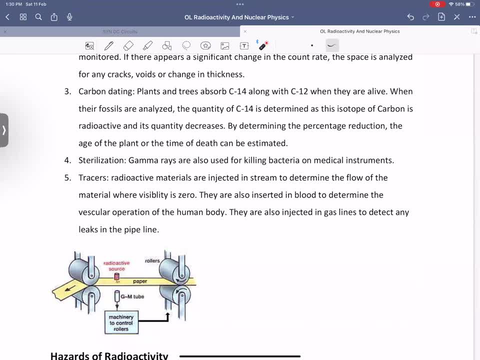 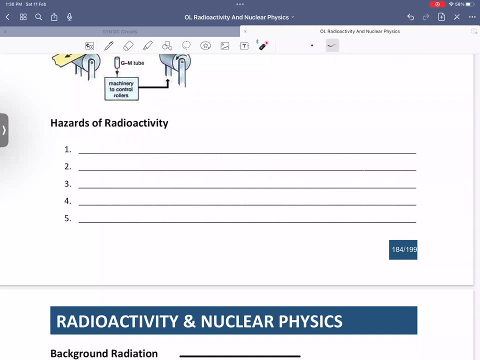 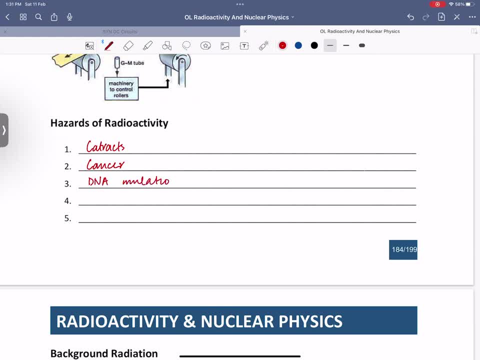 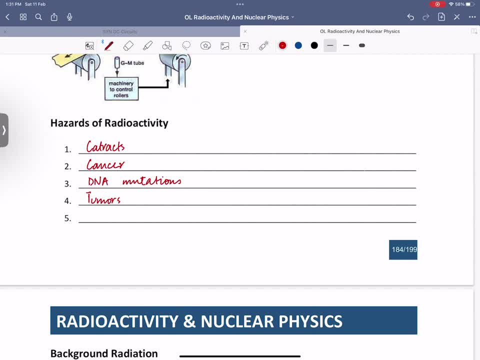 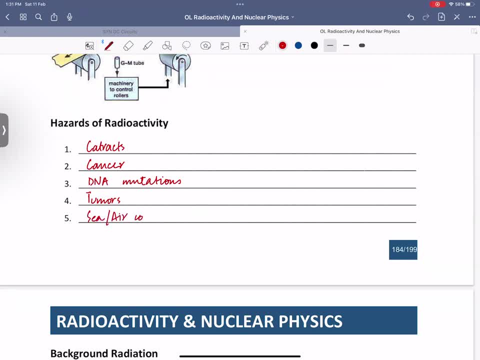 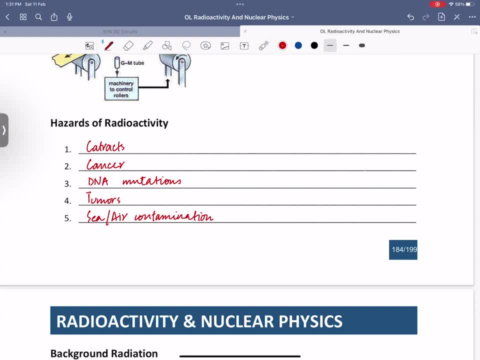 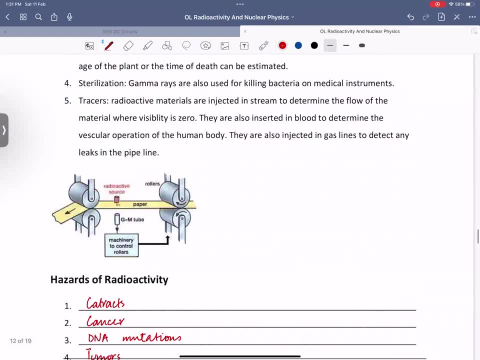 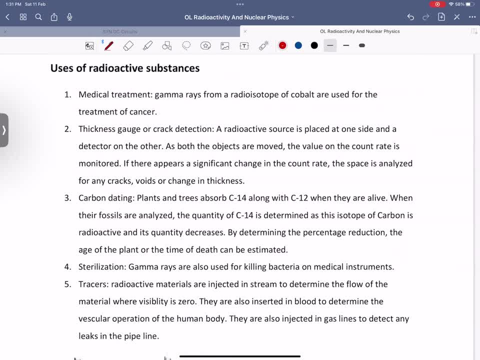 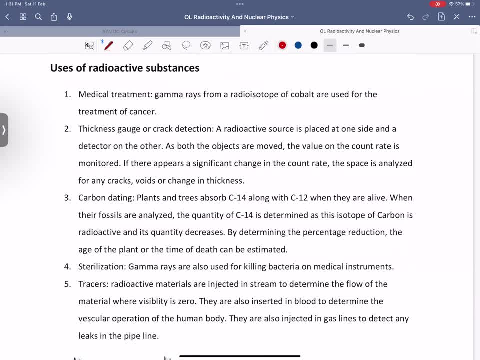 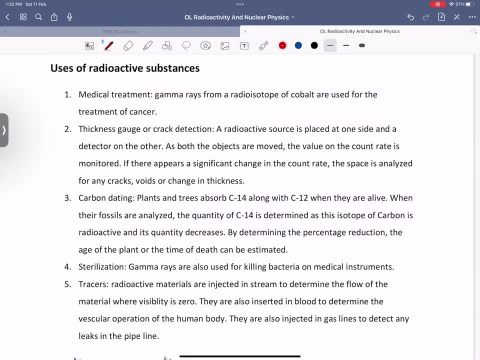 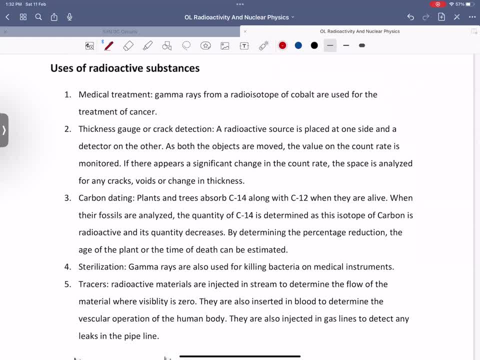 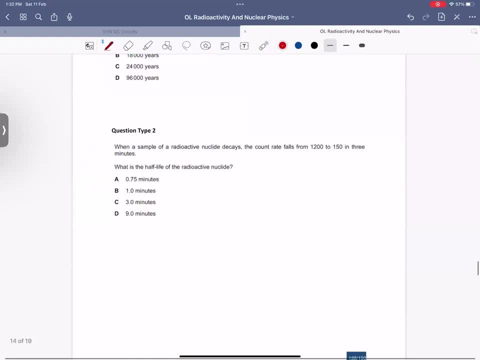 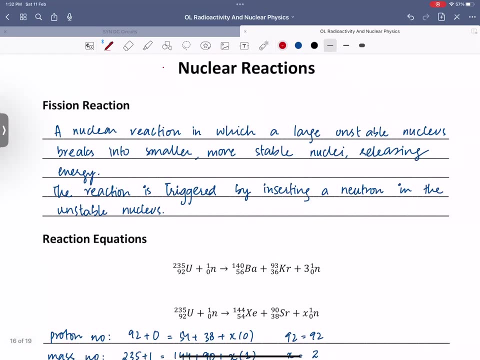 In the absence of radioactivity, you can write cataract, superstBroken, n-delicemen. Let us discuss about nuclear reactions. Let us discuss about nuclear reactions. There are two types of nuclear reactions: Fusion and fission. Fusion is a reaction. 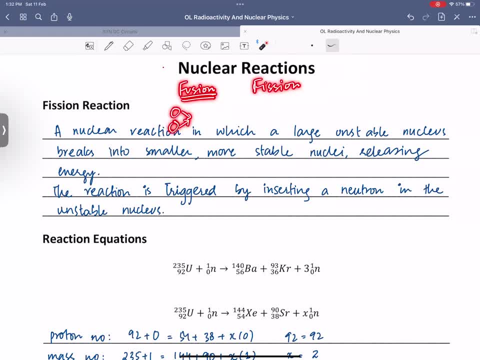 when two small nuclei join and form a larger, more stable nucleus, whereas fission is when a large, unstable nucleus breaks into smaller, more stable nuclei. in fusion your nuclei fuse- they join together- and fission- they disperse, they break down into smaller fragments. both you get questions. 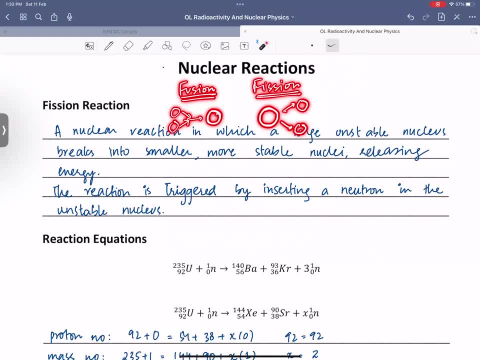 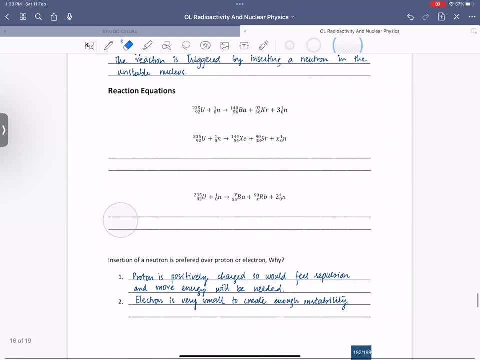 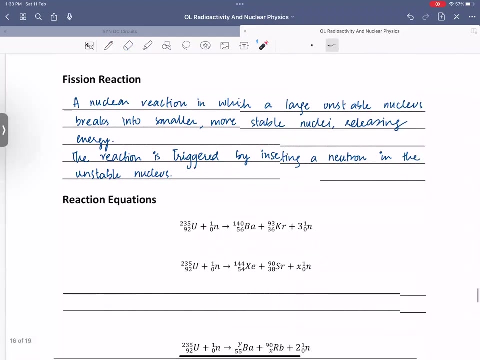 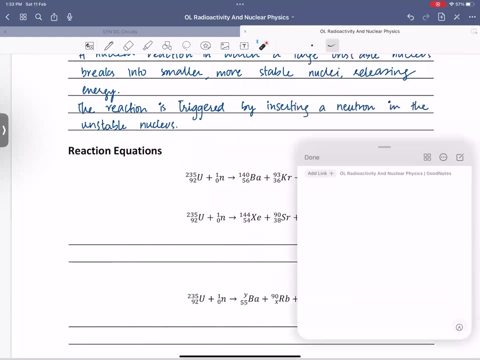 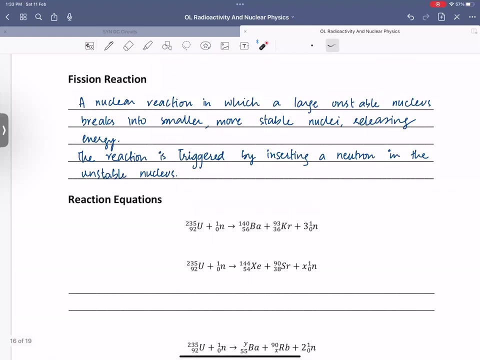 but if you ask, based on energy, we are trying to harness as much energy as possible. first let's talk about fission reactions. in fission reactions, in fission reactions, a large nucleus generally is a radioactive nucleus- see a large nucleus. generally, a radioactive nucleus is already unstable. 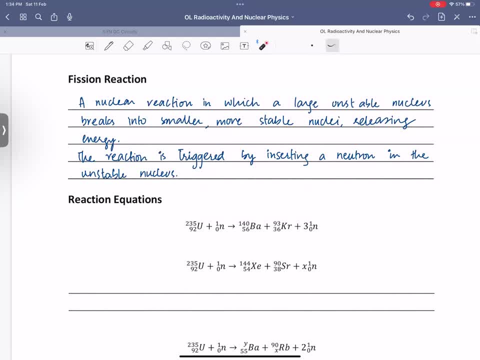 so a large nucleus breaks into smaller, more stable nuclei, releasing energy. there is a nuclear reaction in which a large, unstable nucleus breaks into smaller, more stable nuclei, releasing energy. if you want a definition of fission reaction, you can define it as this. again, this reaction doesn't happen on its own. 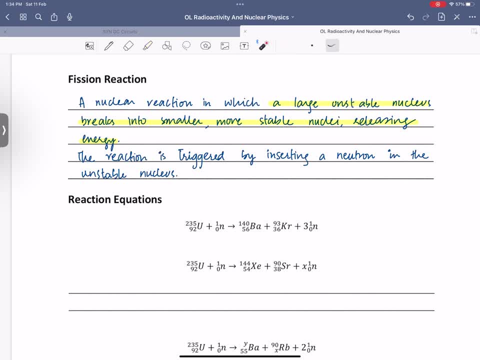 you have to initiate it, and the reaction is initiated by inserting a slow neutron inside it. so a neutron is used to trigger the reaction. a neutron is used to actually trigger the reaction, actually trigger this reaction, because, look, the thing was the uranium, or the nucleus with which you 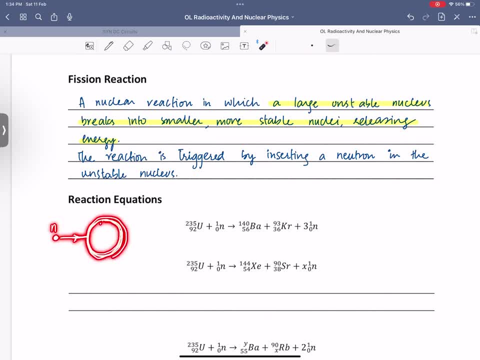 are going to do this fission reaction. that nucleus is radioactive means it was already unstable. all the particles in it were holding it. you inserted a neutron in it, so what happens is that nucleus cannot hold an extra particle and it bursts out into its smaller fragments. it breaks. 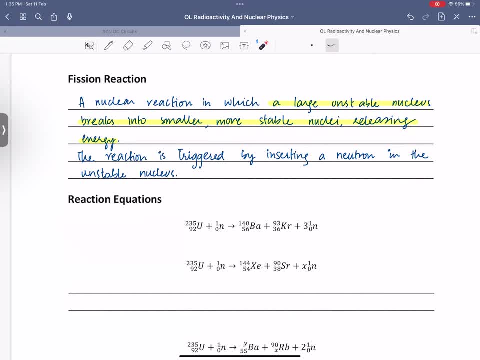 into small atoms and in this process, when it breaks into small atoms, a lot of energy is released, which energy you use in the form of heat and you use it in your power stations, or, if there was a big problem, you could make bombs. so this reaction is: 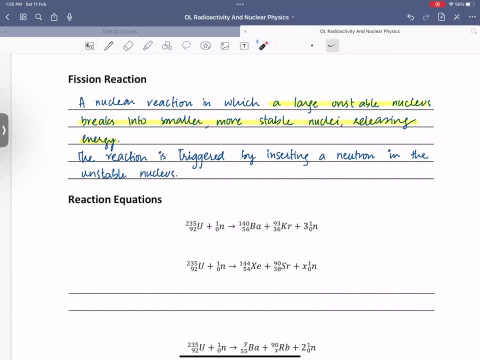 triggered by inserting a neutron into the unstable nucleus. examiner can expect us to kind of like balance an equation. imagine this reaction is given to you and it's one of the fission reactions that actually can happen. you got uranium 92 to 35 and you inserted a 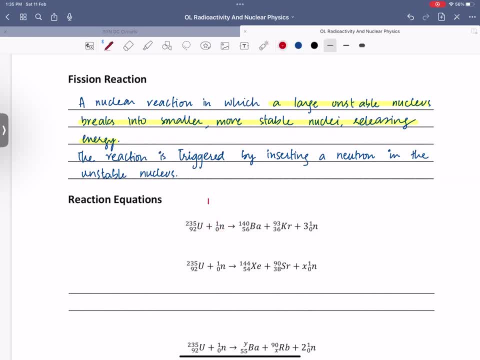 neutron. inside neutrons have a proton number of zero. obviously there are neutrons, they don't have any proton with them. but the mass number is one, because mass number is the sum of protons and neutrons. so the neutron has its own mass number, one. now when 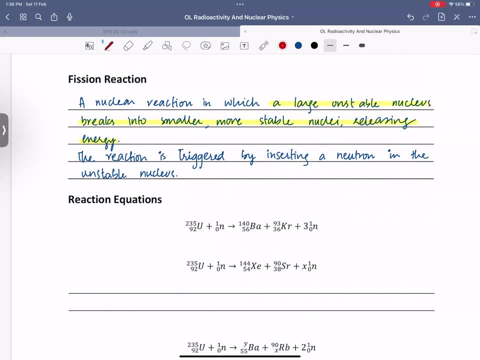 a uranium nucleus receives a neutron, it breaks down into three parts: barium, krypton and three more neutrons. now you don't need to remember. yes, a uranium will break into barium and krypton. you don't need to remember any of it, see, but what? 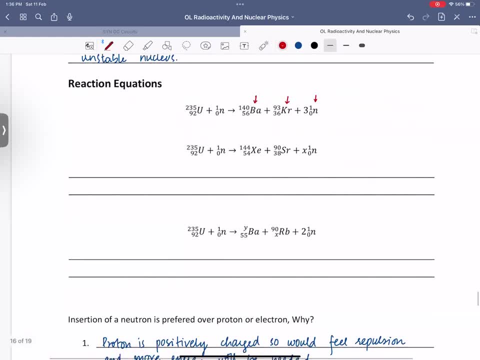 examiner expects us to do is to be able to balance. for example, an equation was given just may: a uranium, when inserted with a neutron, breaks into xenon, strontium and x number of neutrons. see and x number of neutrons. now what happens to find? 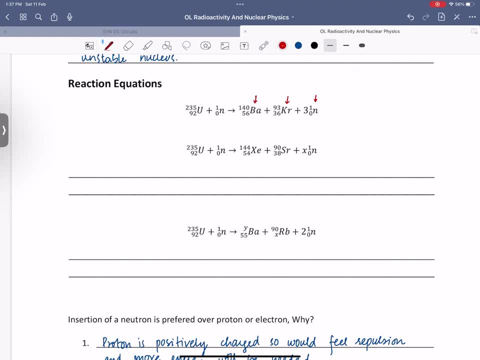 out the value of x. mass number is the mass number conserved in any nuclear reaction. mass number is conserved. proton number and mass number: both are conserved. if i use a mass number, i'll say 235 plus 1. this is the mass number on the. 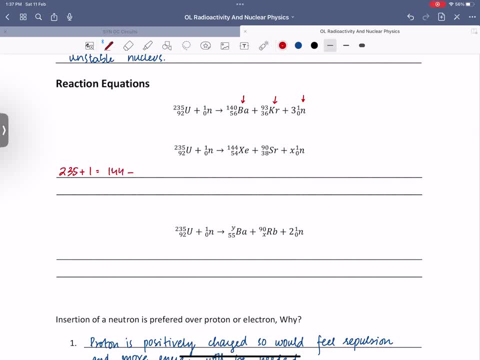 reaction side: 144 plus 90 plus x into 1. this is the mass number on the right hand side: 144 xenon, 90 strontium and i have like x neutron. now what i can do is i can add these numbers up. they're like: 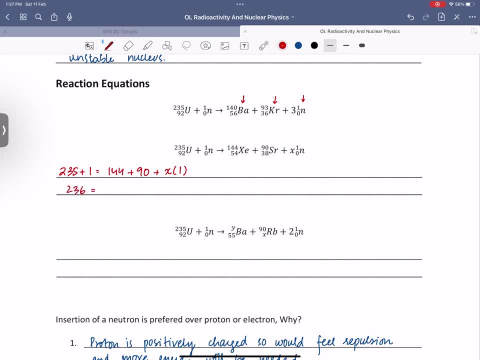 236 equals to 144 plus 90, 134, 234 plus x. so x turns out to be 2 means in this nuclear reaction you're going to have two neutrons produced. so remember that you don't need to figure this number out, so you: 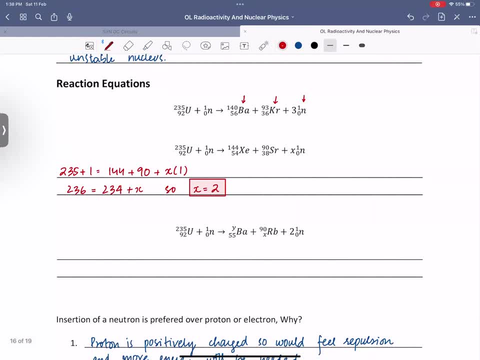 need to know how to figure this number out: proton number and mass number. both are conserved. now i want you to try out this technique on the equation written below and try to figure out the value of x and the value of y. fusion releases the most. now we'll. 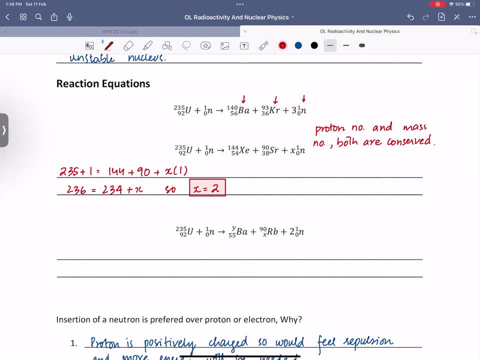 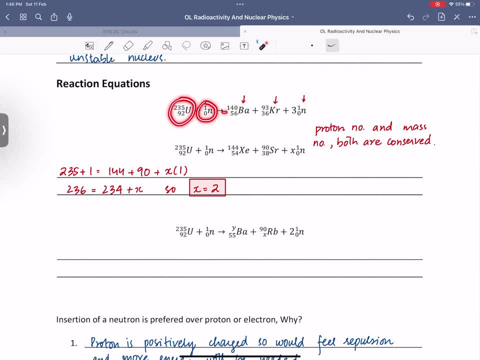 reacting with a nucleus and in turning into two different nuclei and a few amount of neutrons after the completion of slivers with a fog. see give me to you figure out the value of Y and X mass number, the use that give I Miloga, 235 plus 1 equals Y plus 90. let's do neutrons, but you have some. 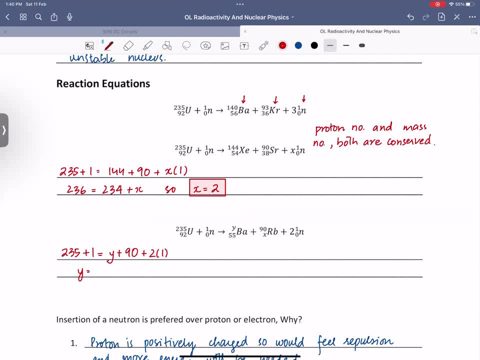 common yoga, that would have been 236 minus 90 minus 2. Y would have been 140. is it a proton number you use? turkey affects me now: 92 plus 0, 55 plus X, whopping you're talking about two into zero. he got it off, I, then he. 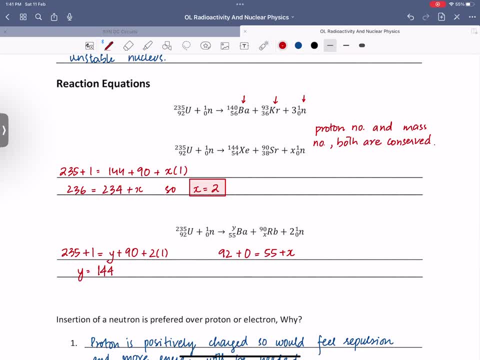 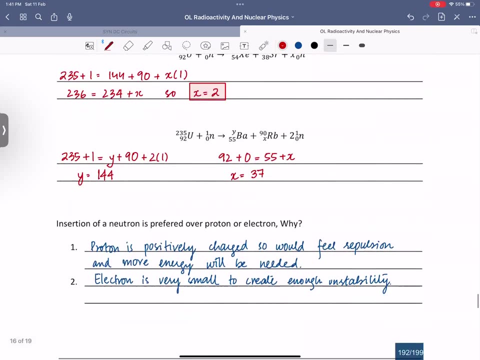 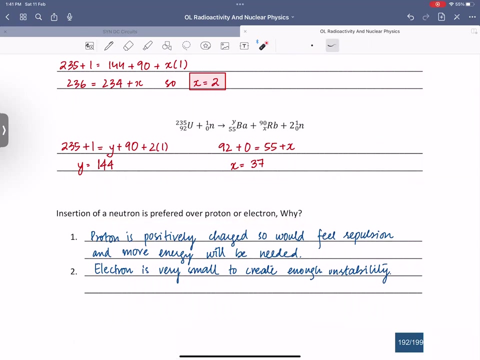 will be: 92 minus 55 gives me 37. you're gonna have equations like these for your questions. stupid, that I mean. why do you prefer inserting a new phone rather than a proton or an? there are simple reasons. they go proton basically. a proton is a. 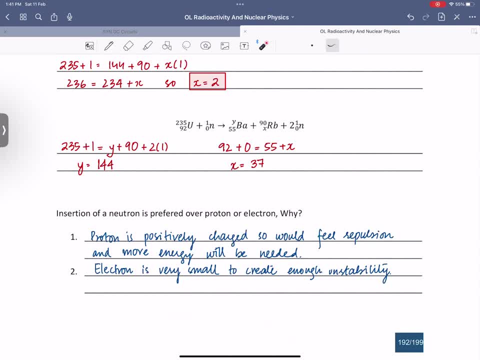 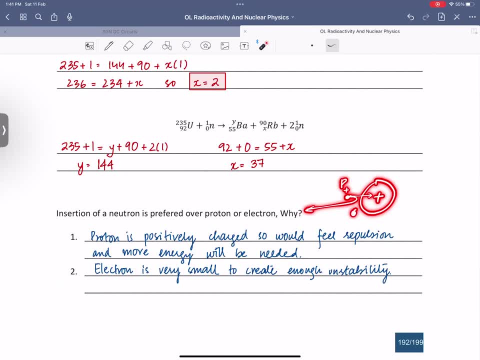 licking neutron. it's of the same size approximately and if you tell it's easier for a neutron to get into a new zicharani and then J rechtically more feasible to use up neutron. the symbol as shown in the evaluation pack number 3 is not available in a uci. mutants thrown away so that you might not get any torpedo, that if you mean one breaking through a group, you may lose energy or hopefully even substitute using a neutron nap, which is a electron. you cannot use there una fraga and". Second, the issue with electrons is that electrons are very, very small. 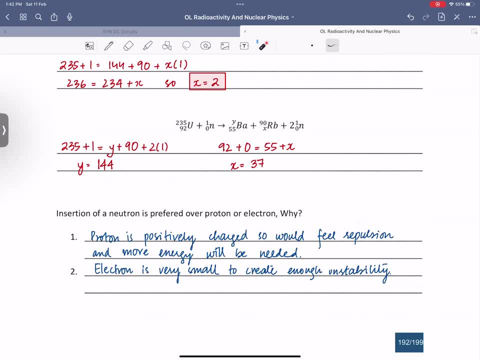 They don't actually have that much of a mass that can make the nucleus unstable And, besides, electrons don't have that force that is needed to bind the nucleus Electrons don't experience that. I had taught this in beta particles And I told you that when an electron was produced along with a proton, 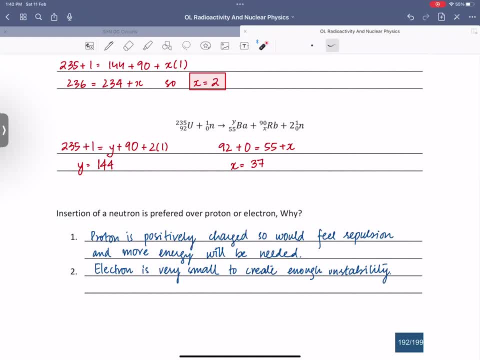 the nucleus held the proton inside. The electron didn't hold it. The electron came out As a beta particle, So the force that holds the nucleus doesn't experience the electron. You were inserting particles inside so that the force would be a little bit worse. 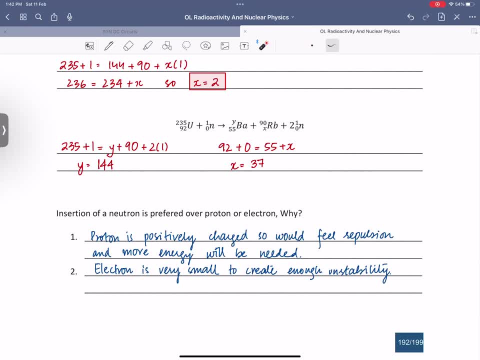 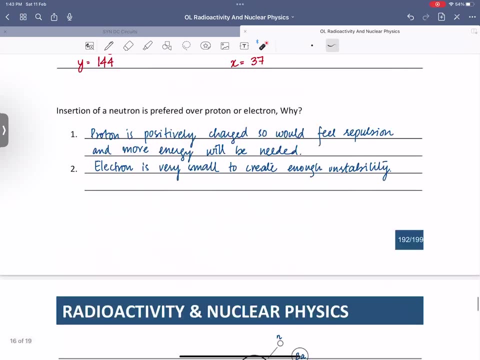 The particles were able to hold it. You have to send the particles inside. That's why you prefer sending electrons. Although it comes to mind that it is negatively charged, It will attract, But you don't do that. Yes, there is a chain reaction that you need to know about. 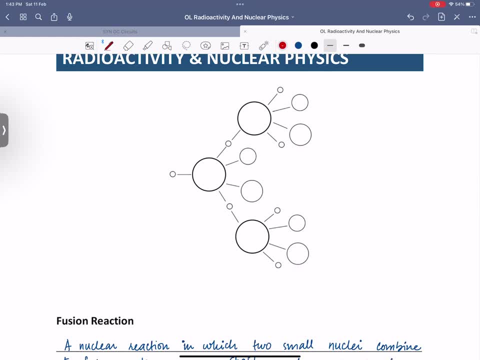 The chain reaction is basically how a fission reaction works. After initiating a fission reaction, you have to control it a little, Otherwise it increases at an uncontrollable rate, Because it is a chain reaction. Chain reaction means that the products created at the end of this reaction 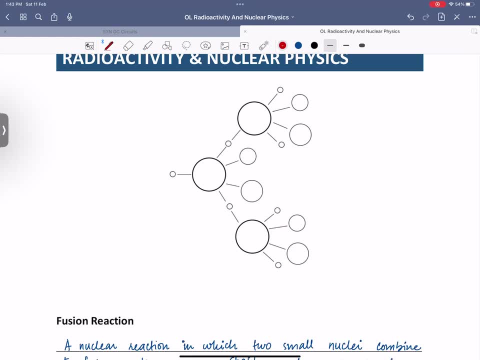 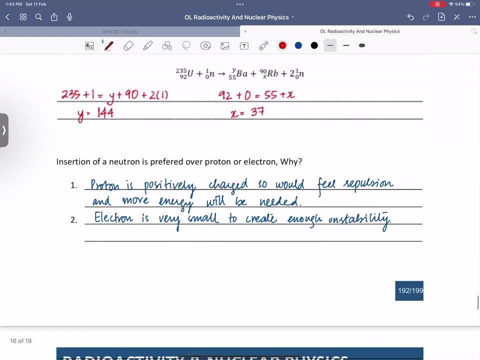 those products promote this reaction in a way. What I mean to say is that the neutrons inserted in uranium were broken, And let's say they break. Let me take an example here. It was converted by barium and krypton. What happened? 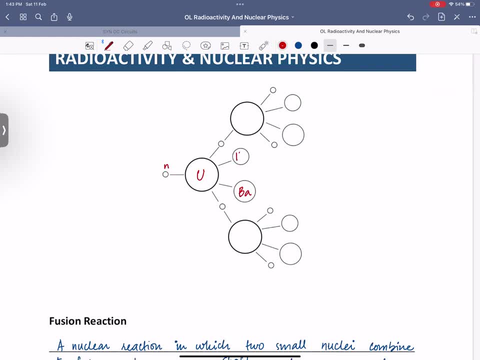 It was converted by barium and krypton. What happened? What happened? What happened? I call it any element xy, Any element converted into x and any element converted into y. You don't need to worry about it at the moment. But in addition to this, it also makes some neutrons. 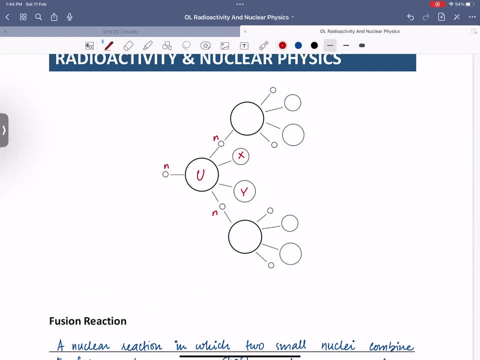 Like I made two neutrons here. At the end of this product those particles are also created which are used to trigger this reaction. To trigger this reaction. Now. there is not going to be one atom of uranium in a lump of uranium. 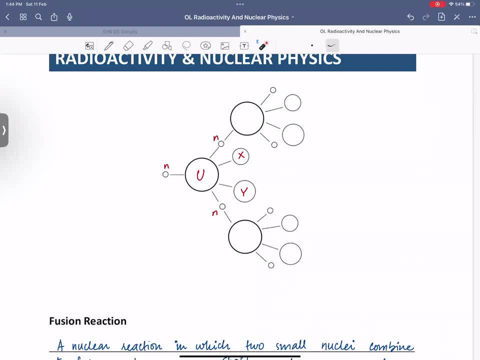 There are going to be like trillions and trillions atoms of uranium. So you initiate a reaction in one and the reaction propagates on its own. If one uranium breaks, the neutrons that will be produced, these neutrons will actually cause the other uranium. 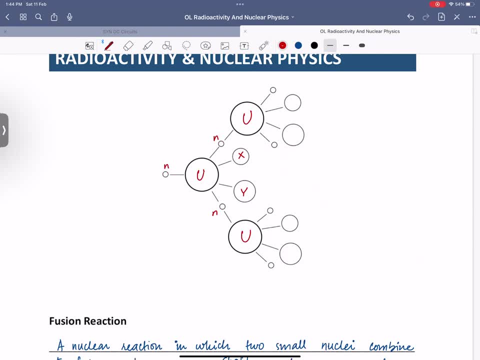 atoms to break as well, These other uranium atoms will be inserted, and when those uranium atoms break, they will also produce neutrons. So these neutrons will actually trigger reactions even further and it's like a chain reaction. It will keep on going And it will increase at an uncontrollable rate. 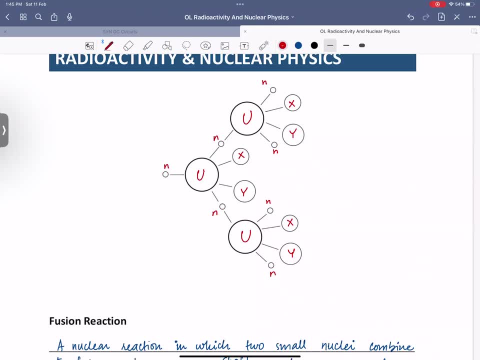 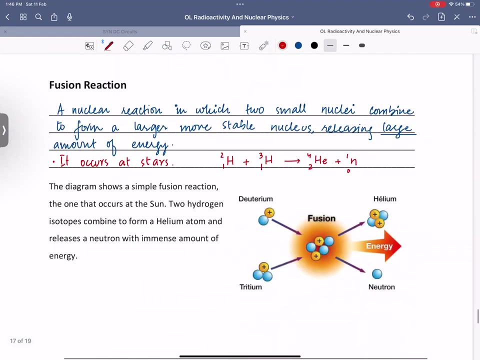 So in our power plants in which we produce energy through nuclear fission reaction, in those power plants we have to control this reaction. We will talk about how it is done later, But we have to control how it is done later. On the contrary. Yes, I was not saying anything. 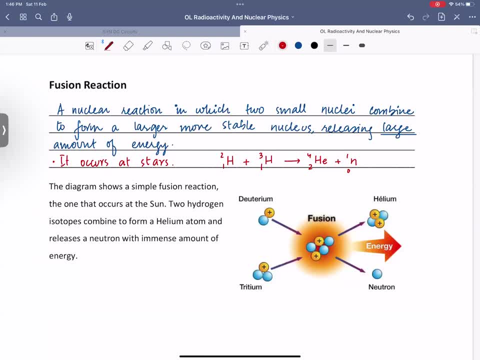 I was quiet. Okay, Now let's talk about fusion reaction. When we talk about fusion reaction, then in fusion reaction the reverse happens. You don't break a nucleus into smaller fragments, You join smaller atoms and make it into a larger one By joining small. 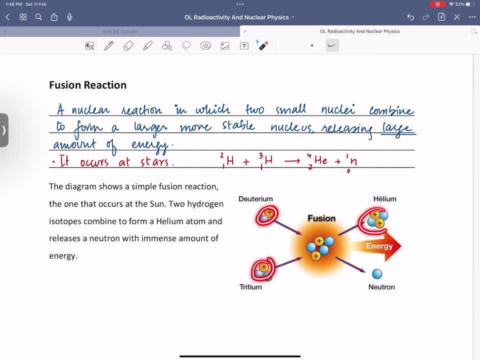 nuclei, a big nucleus is made. That's why it's called fusion, derived from the word fuse- Join, See the word fusion is derived from fuse And fuse means to join. So it's a nuclear reaction in which two small nuclei combine to form a larger. 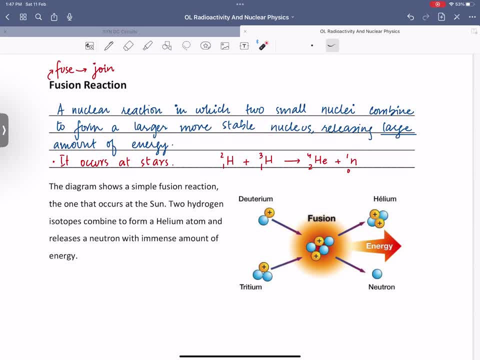 more stable nucleus. But when you write this definition, the examiner wants one thing to be clear: He wants you to use the word in releasing large amount of energy. It generally happens with two small nuclei, Not with more than two, Releasing a large amount of energy. 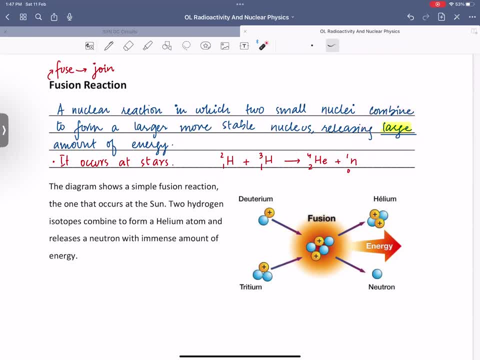 Emphasis is on this word because this word, in comparison, tells us that the energy of this reaction is more than that of a fusion. This reaction produces more energy than a fusion reaction does, And it occurs actually on the stars, Because the energy required to create this reaction 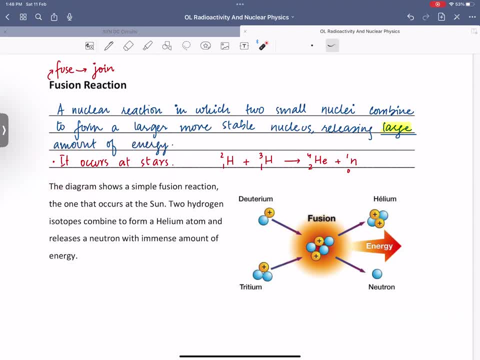 cannot be created on earth as such. To join two nuclei- both are positively charged, See. to join those two nuclei and make a large nucleus, See, it's not energetically possible. The high temperatures you need to conduct this are usually formed at the start. 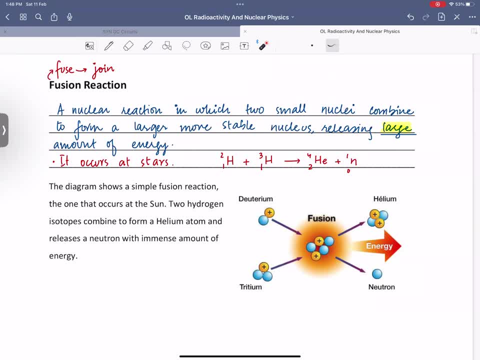 That's why even our sun has a nuclear reaction. There's a nuclear reaction going on in it, Even in that the hydrogens are combined to make helium. And which are those hydrogens? They are basically deuterium and tritium. 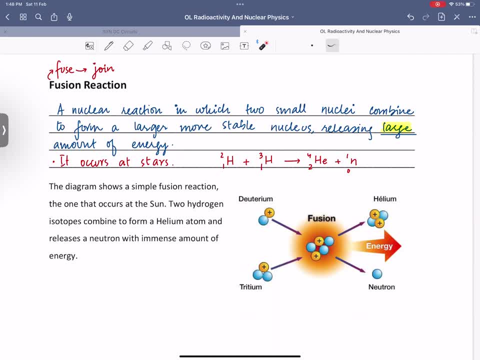 These are the two isotopes of hydrogen that are joined Because deuterium is 1,2 and tritium is 1,3. They join and form a helium atom, A helium nucleus, 2,4, and one neutron is released. 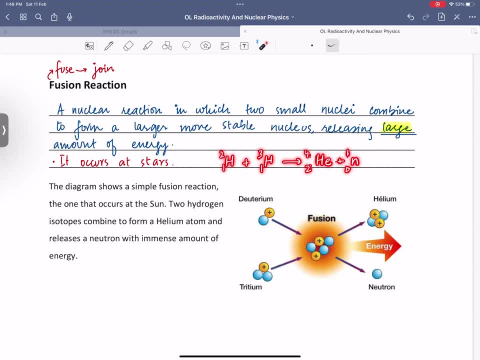 So, but this reaction is not a chain reaction. This reaction is not a chain reaction. You're not breaking atoms, Or you're not breaking nuclei, So you're joining them. So this neutron has nothing to do with the next reaction. 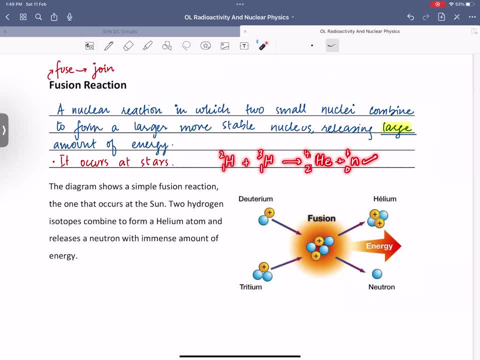 It was in fission. The neutron that was formed in the product was used as a fuel to start the next reaction. This was the result of the radiation reaction. They were able to do that. Yes, my dear children, Energy is released in both of these reactions. 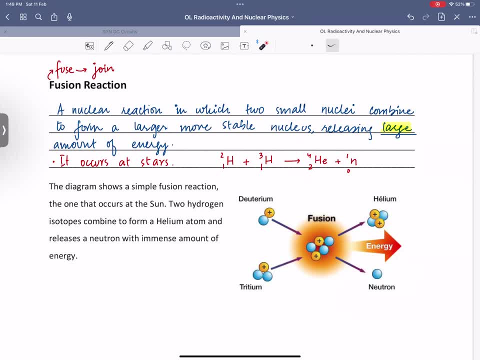 But if we talk about the energy requirement, fusion requires more energy. That is why fusion releases more energy, But it's way more than you actually need. No, but it doesn't need a proton. it's a fusion and it has to be joined. 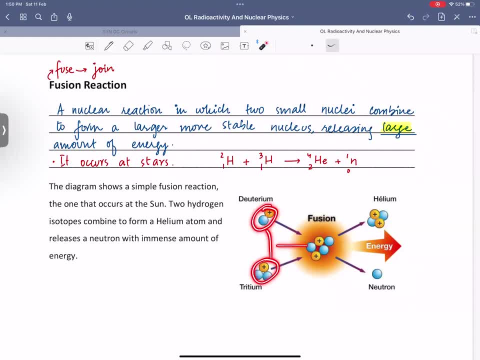 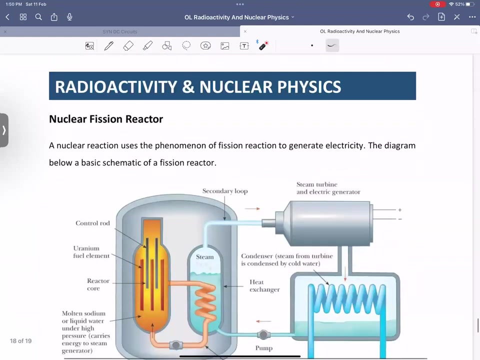 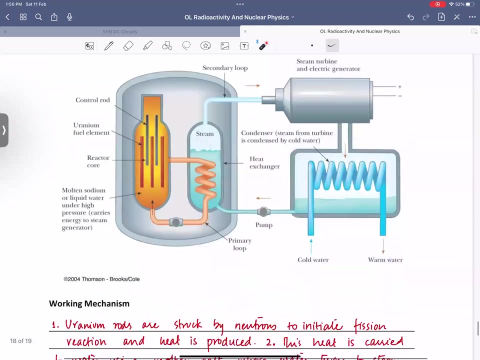 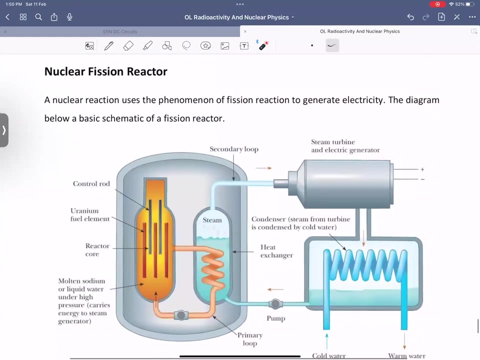 So they themselves- deuterium and tritium- get together at high temperatures and convert into helium. Then we've got a fusion reactor with us. It's been a while since examiner has actually asked about a fusion reactor, Whether fusion reactors, how fusion reactors work or not. 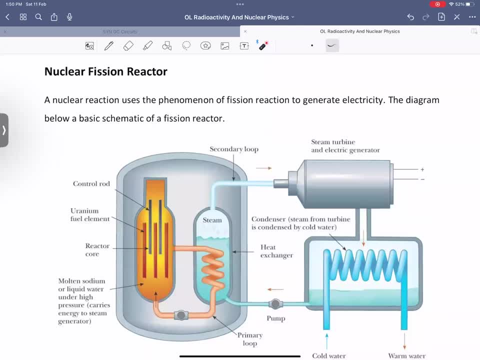 Let me check if it's still in the syllabus or not. If it's not, then it won't be of any use. But if it's there, then we'll study it. If it's not, then we'll study it. 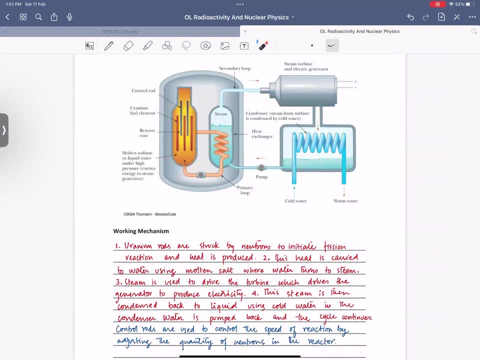 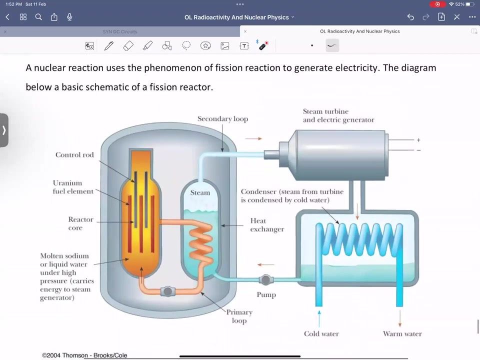 If it's not, then we'll study it. I want you guys to give it a read first. When I'm explaining, you guys can process what's going on over there. I want you guys to give it a read first. When I'm explaining, you guys can process what's going on over there. 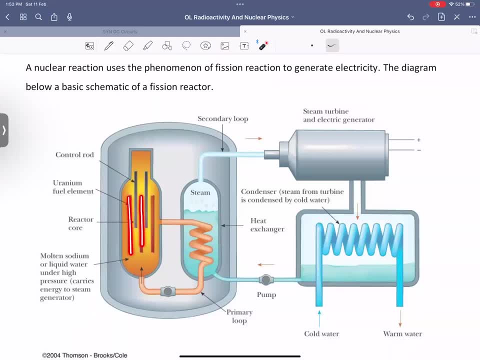 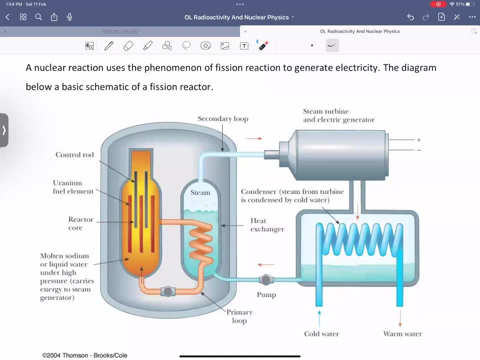 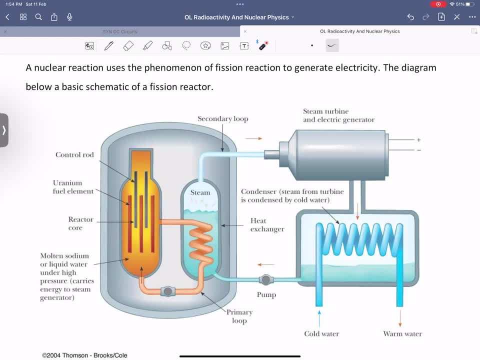 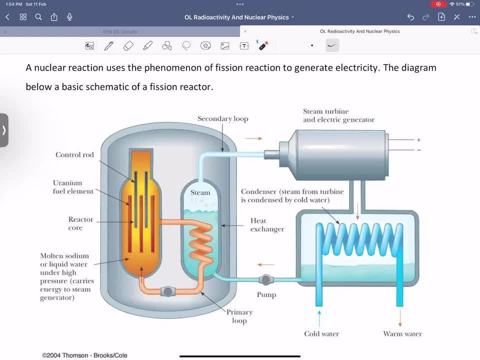 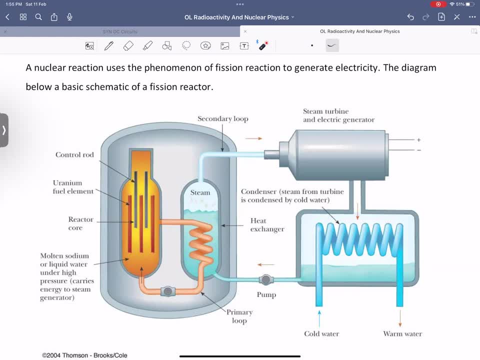 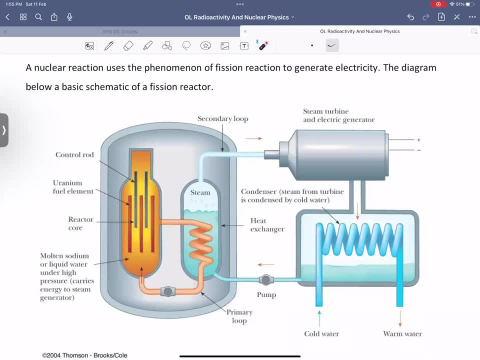 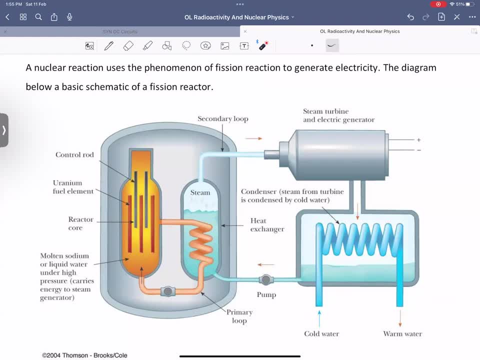 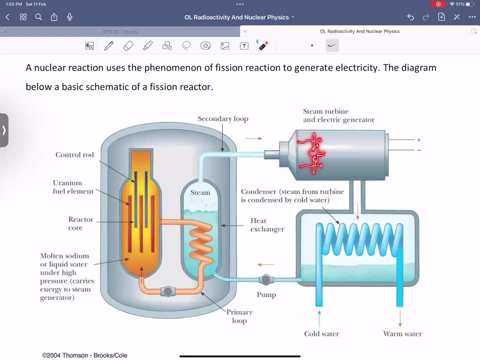 where it hits the steam and rotates the turbine. The rotating turbine runs your generators, Where you get electrical energy from, And the steam returns to the condenser. And the steam returns to the condenser. Actually, we need steam because we need to run the turbine. 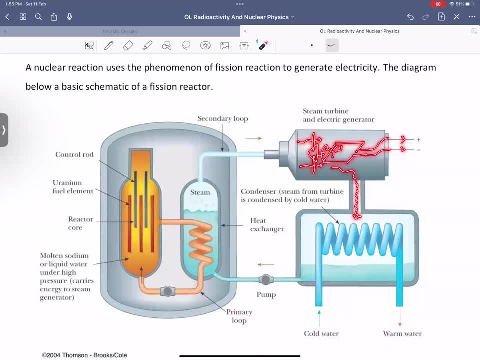 Just like the wind turns the turbine and the falling water turns it, similarly we want to turn the turbine through steam. So when we hit the turbine blades with the help of steam, the rotation was created. That rotation rotated our coil, which gave us the current. 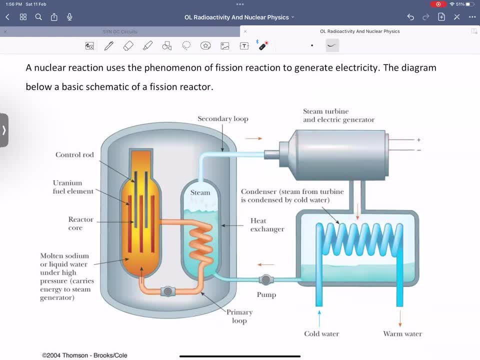 And the steam went back to the condenser. Condenser, as the name suggests, is condensing the steam to the form of vapors. For this you take cold water, which is usually taken from the sea. That's why you attach these power plants near the sea. 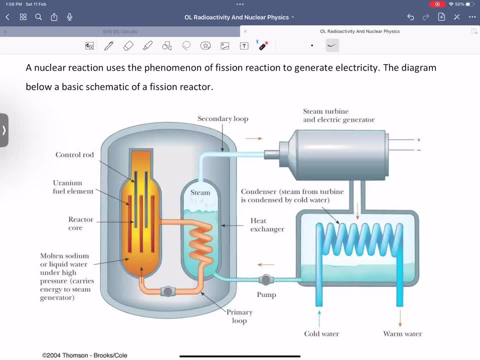 So, usually from the sea, you put the cool water in your condenser. The steam condenses on it and becomes liquid, And this cool water gets a little warm and goes out. It is then disposed back into the sea And this steam, which was also made of liquid, 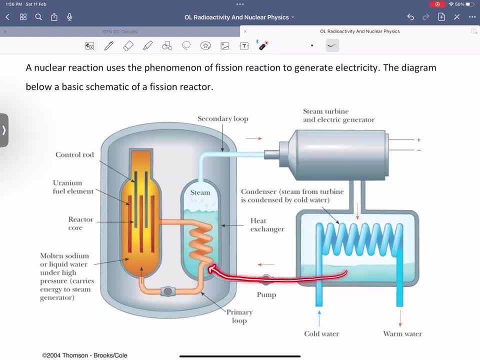 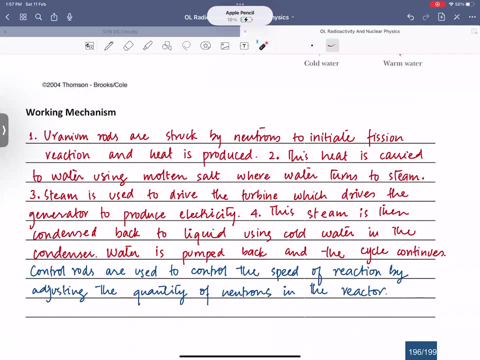 this liquid goes back to you. It is then pumped into this container So that the cycle continues. This is what we have written in the wording: How your uranium rod is struck with a neutron and the fission reaction occurs. You make steam out of the heat that comes out of it. 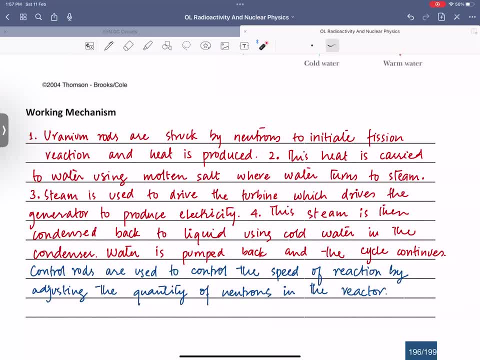 Steam hits the turbine blades and it turns your generator to produce electrical energy. This steam is condensed back and sent to your container, where it came from, So that your cycle can be repeated again. So we'll be keeping the lesson till here. Inshallah, in tomorrow's class we'll be completing radioactivity.